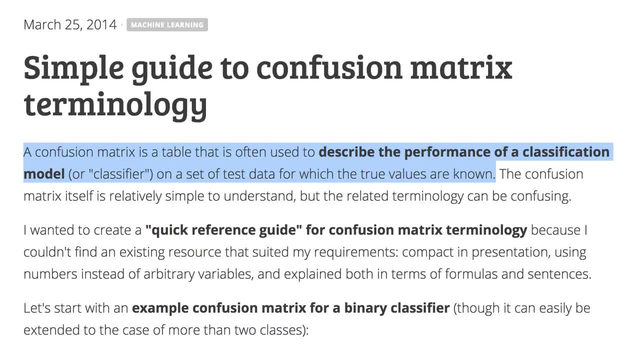 on a set of test data for which the true values are known. So two points I want to highlight here. Number one is that a confusion matrix is only used for classification models, meaning models that are predicting class labels, and they are not used for regression models meaning 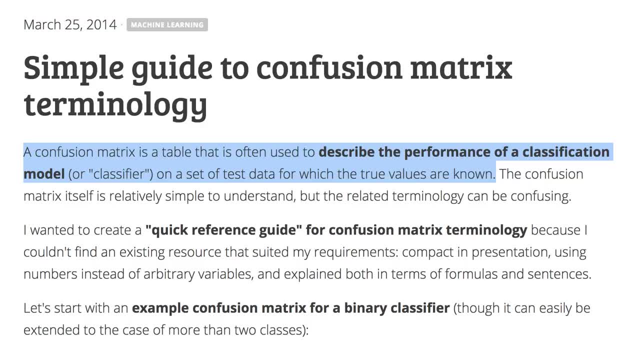 models which are used to predict numeric values. The second point I want to make is that the confusion matrix can only be computed when the true values are known. meaning, if you've used an evaluation procedure like train-test-split, then you do have a set of test data for which the true values are known, and when you make 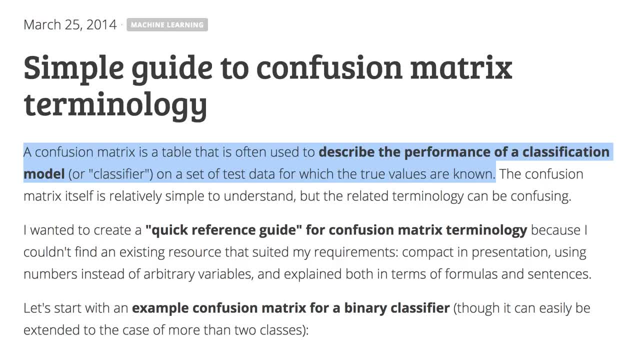 predictions on that test set, you can use a confusion matrix to evaluate them. Alternatively, if you are making predictions on out-of-sample data for which you are able to eventually measure what the true value was, you can also use the confusion matrix. Let's go ahead and pull up an example confusion matrix that I've created and we'll talk about. 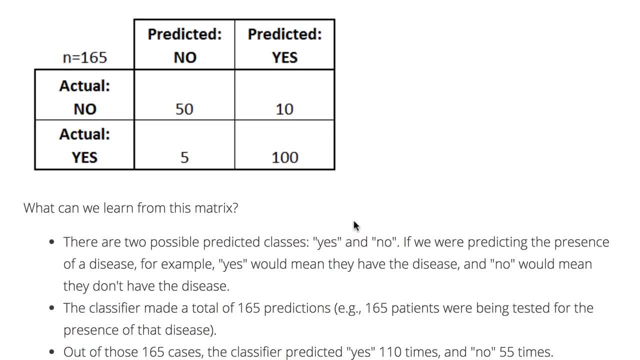 what we can learn. You'll see that there are two possible classes in this case, which is why it's a 2x2 matrix. If there were three possible classes, then it would be a 3x3 matrix, and so on. 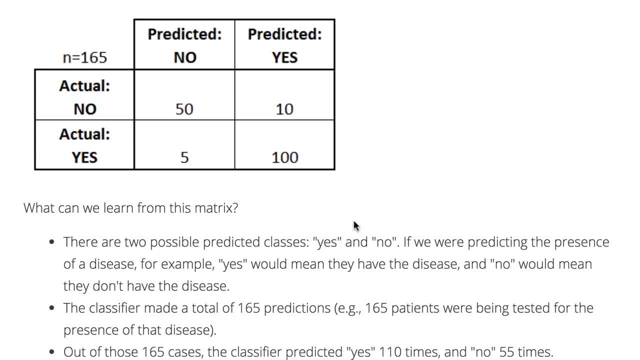 In this case, the two possible classes are no and yes, but they could be other things like 0 and 1, or blue and green, Or really anything. We can tell from the confusion matrix that it made a total of 165 predictions, and we 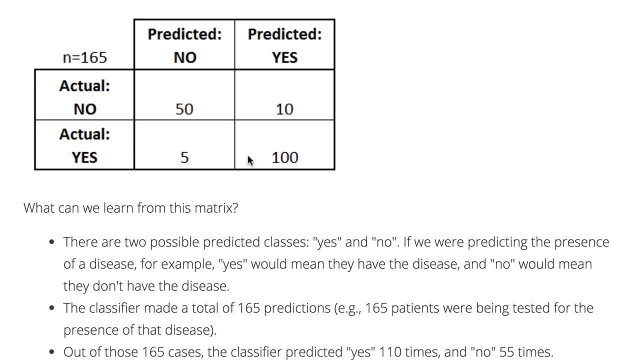 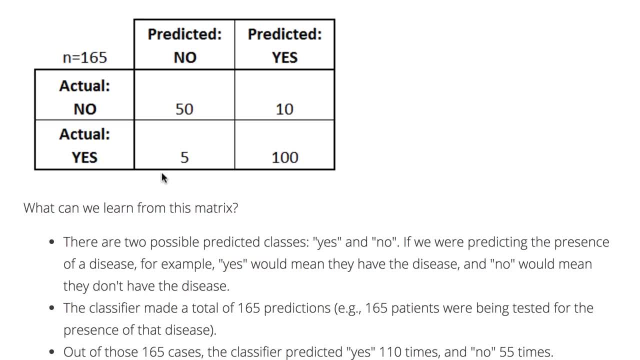 Well, there are four terms we're going to go through To start. these 100 are called the true positives. So these are cases. 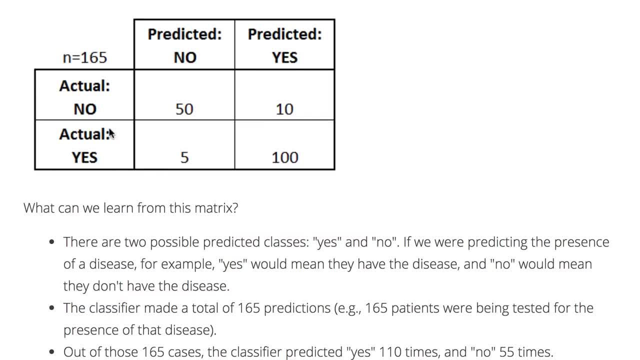 in which the actual value was yes and the predicted value was yes. these were called true positives. There were a hundred true positives. These are called true negatives. These are cases in which the actual value was no and the predicted value was no. 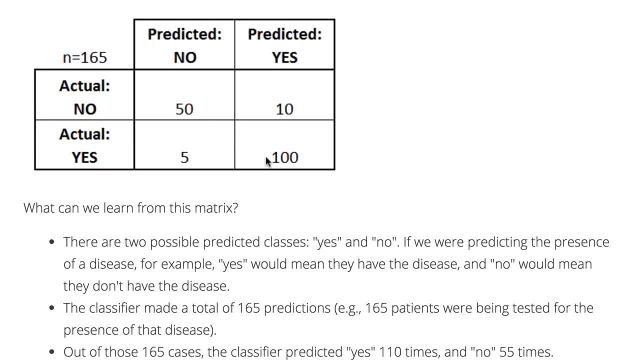 So both of these are numbers that you'll always want to maximize. Okay, now the third term is called false positives. This is a case in which we have the actual value is no and we predicted yes. Again, these are called false positives. 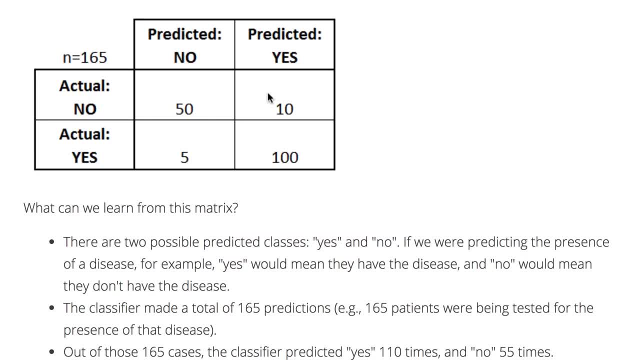 and the way I remember them is. I insert the word predicted between false and positive, as in: these were falsely predicted as positive. We falsely predicted the positive class. So yes is the positive class and no is the negative class. So these are true positives, these are true negatives. 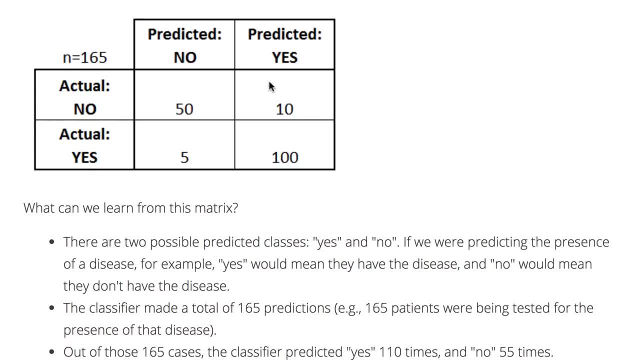 and these are false positives because we falsely predicted the positive class when the actual value was the positive. So this is the negative class. You may have heard the term type one error. False positives are type one errors. okay, Now you can probably guess what this fourth box is called. 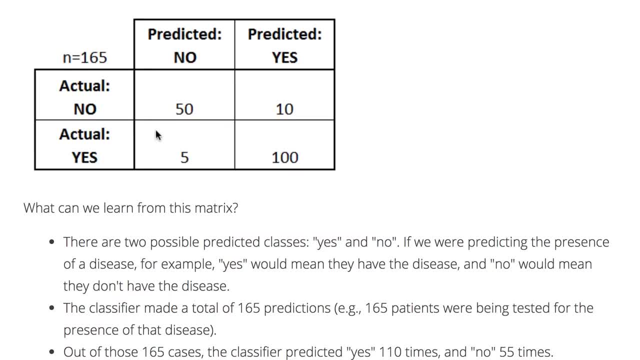 These are called false negatives. These are cases in which the actual value was yes, but the predicted value was no. So again, we insert the word predicted between false and negative, to remember it. and false and negative are false positives. False negatives are when you falsely predicted. 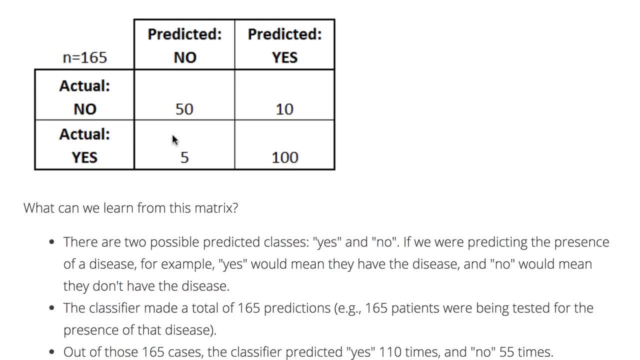 the negative class. You predicted the negative class and you were incorrect. okay, These are known as type two errors. Not everyone uses that terminology, but it's common in the scientific community to talk about type one errors and type two errors. Now, before we move on, 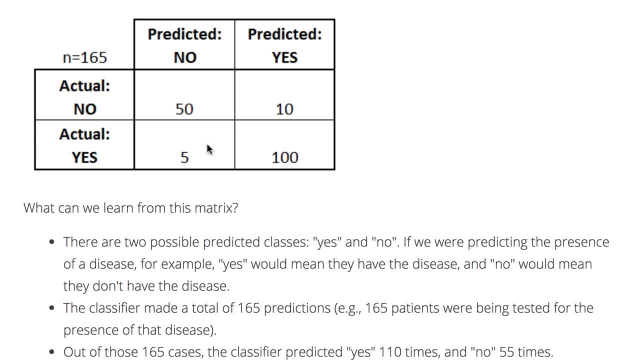 there are three important points I want to make. Number one, and probably the most important, is that when we talk about true positives, true negatives, false positives and false negatives, these are whole number counts. You can think of this as a tally, okay. 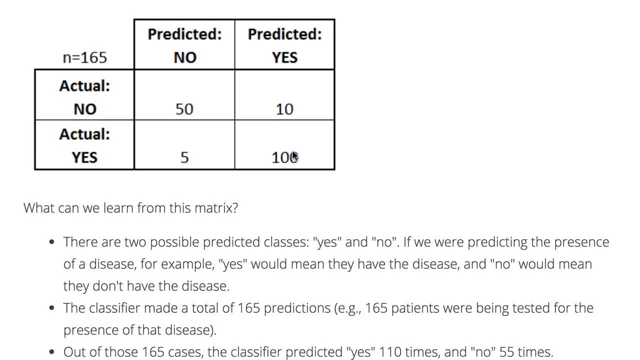 A cross tabulation. These are not rates, These are not percentages, There are no decimals When we talk about those numbers, the true positives, et cetera. those are whole numbers, They are a count. There were 165 predictions. 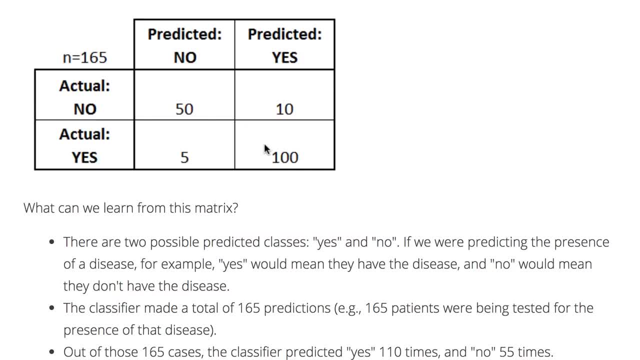 and 100 of those times they were true positives, 50 of those times they were true negatives, et cetera. So that's number one. Number two: these terms true negative, true positive, these terms only make sense when you have a positive class. 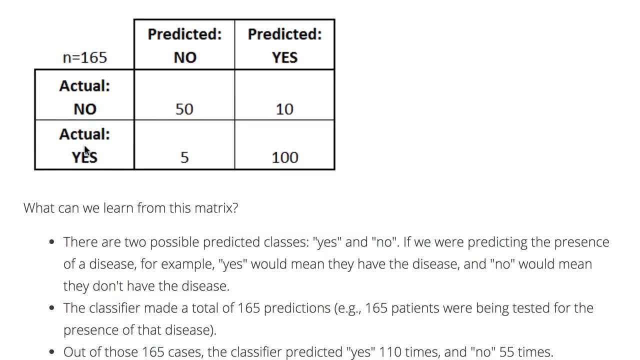 In this case, I defined the positive class as yes and the negative class as no. If you had the numbers, if your class labels were zero and one, you would define zero as the negative class and one as the positive class. If you were building a detector of fraudulent transactions, 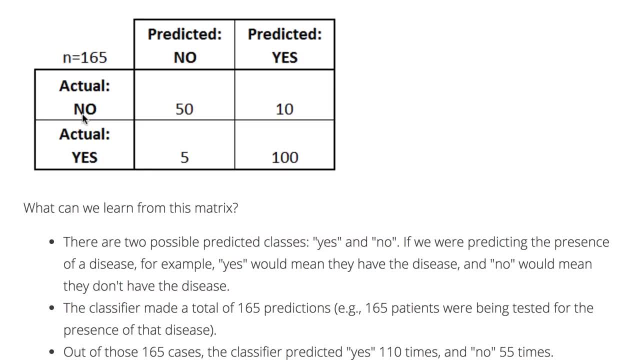 you would define it not fraud as the negative class and fraud as the positive class. That would be the convention. Now what if you had class labels like blue and green, where there's no obvious way of saying what's the positive class and what's the negative class? 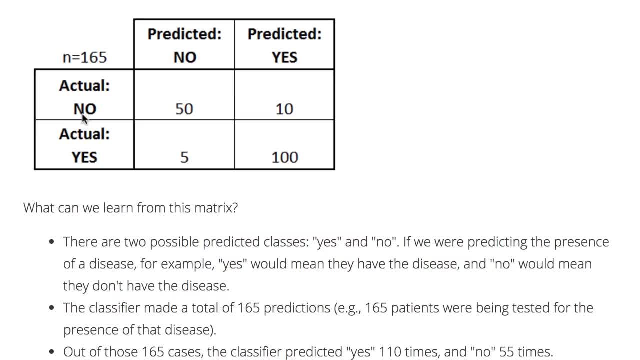 In that case you would just pick and you can be arbitrary of what is the negative class and what is the positive class, and you just have to make sure that that's clear to you and clear to the person reading your confusion matrix. And then point number three before we move on. 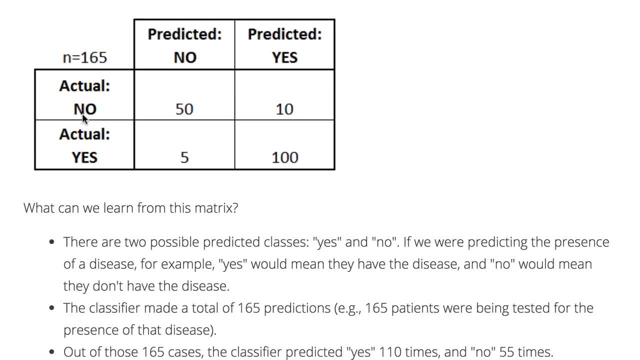 If you have more than two classes. I don't recommend using the terminology true positives and true negatives and false positives and false negatives. Now, some people do this and you can do it if you use what's called a one versus all approach. 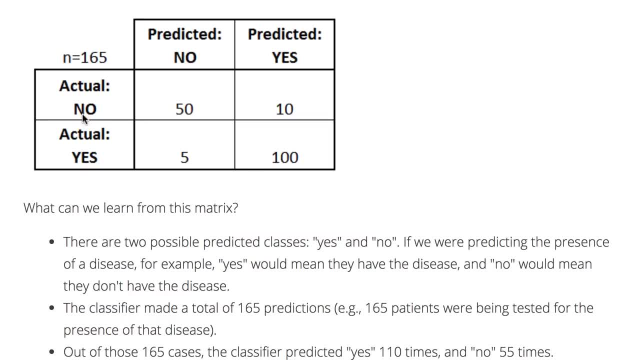 But that is confusing. That's all beyond the scope of this video for me to explain. But the bottom line is, if you have more than two classes, it's confusing to most people to use the terms true, positive, true negative, etc. 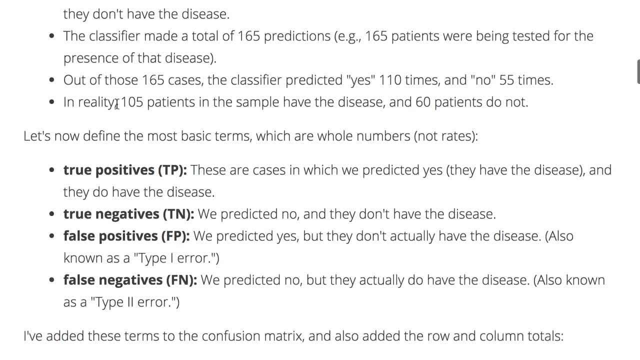 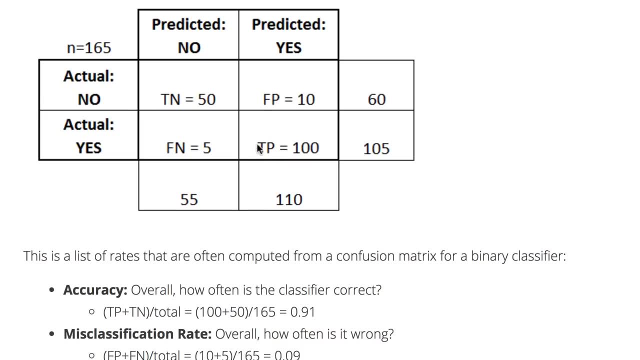 Let's scroll down to another version of this confusion matrix, in which I've added those terms or abbreviations- true positive, true negative, false positive, false negative- and I've also added the row totals and the column totals. Now from this confusion matrix. 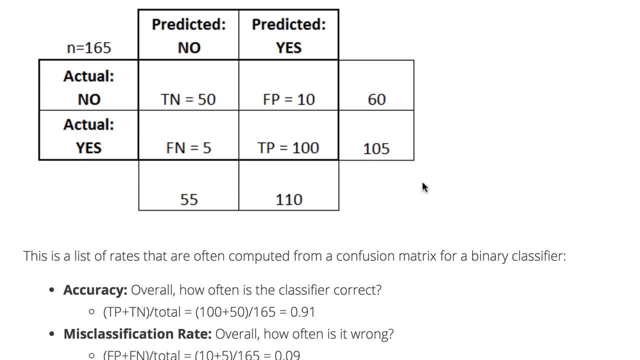 we will compute what are known as model evaluation metrics. These are rates that will help you to evaluate your model. Now, to be clear, the confusion: matrix is a table that helps you to understand your model's performance, whereas the metrics we compute from it. 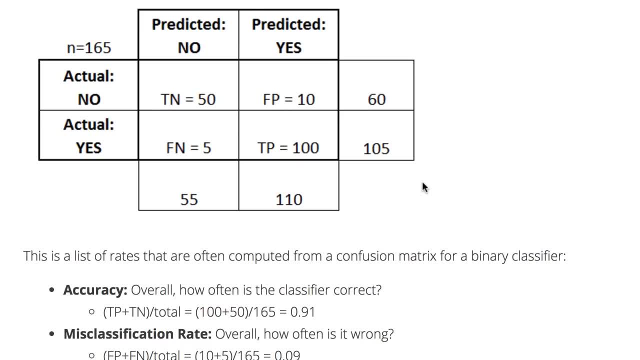 will help you to choose between your models. They're the concrete hard numbers that we we will use to choose between models. The first rate we'll talk about is accuracy, and it answers the question overall: how often is the classifier correct? 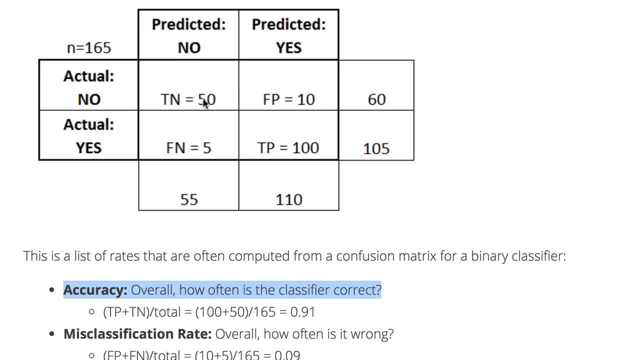 So what we do to compute, that is, we add the true negatives and the true positives, 50 plus 100, and then we divide it by the total, which was 165.. So our accuracy, the classifier's accuracy, is .91 or 91%, okay. 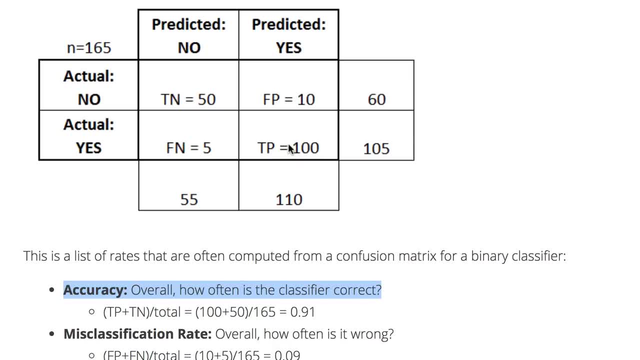 So that's the accuracy. Now the opposite of accuracy is misclassification rate, also known as error rate. You can do it one of two ways. Either you compute. you can compute it by saying one minus accuracy and we would say our misclassification rate. 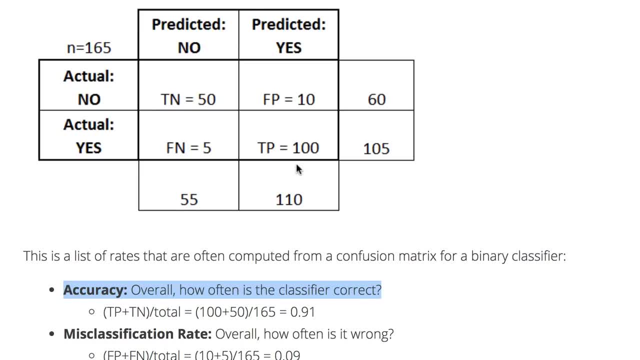 or our error rate is 9% or .09, or we can just compute it directly by saying 10 plus 5 divided by 165, which is again the total number of predictions. So the misclassification rate is .09.. 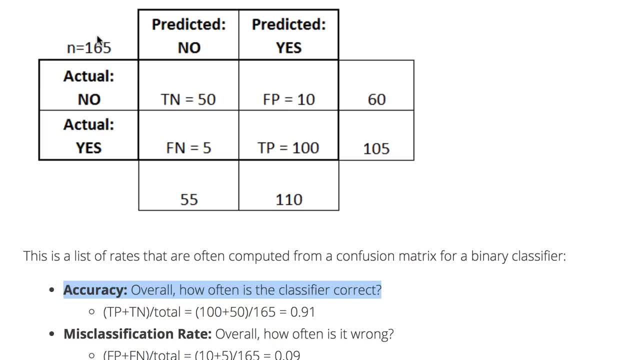 Now thinking about multiclass problems, which are classification problems with more than two classes. let's say you had three classes. the accuracy is computed along the diagonal and we'll see an example of this later- but the accuracy is basically just computed. 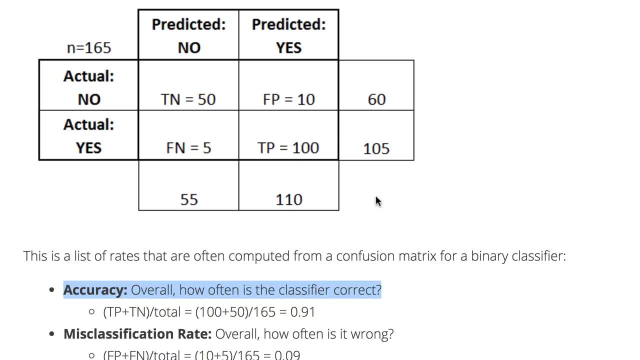 by adding up all the numbers along the diagonal and then again dividing it by the total number of predictions. So accuracy and error rate are model evaluation metrics that extend naturally to multiclass cases. That's not the case for all the rates we're going to talk about. 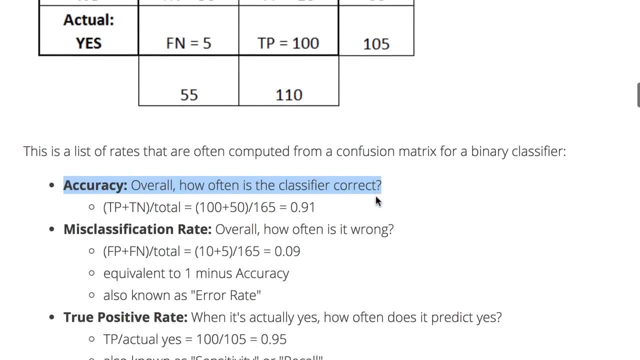 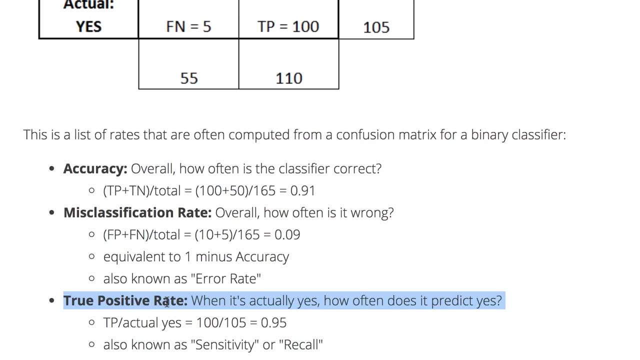 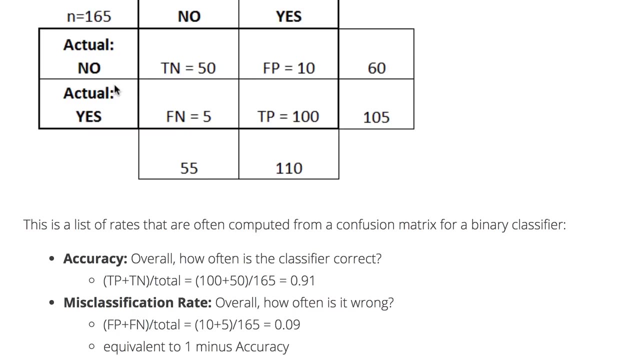 The next rate I want to talk about is called the true positive rate and it answers the question: when it's actually yes, how often does it predict yes, Okay, So when it's actually yes, so this row: 105 cases. 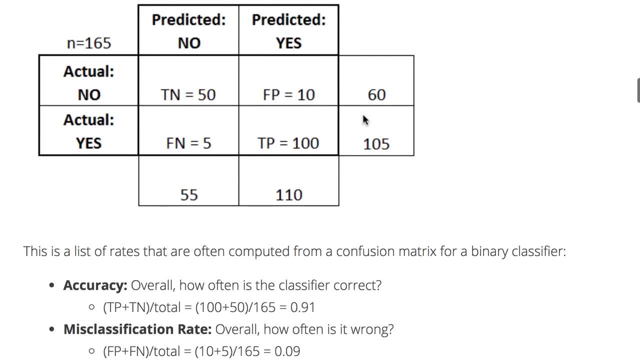 how often does it predict? yes And 100.. So the true positive rate is 100 divided by 105, which is about 95%. Okay Now, true positive rate is also known as sensitivity. That's often a scientific term. True positive rate is also known as recall. 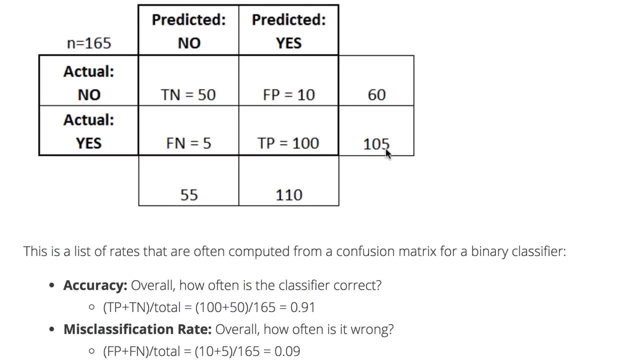 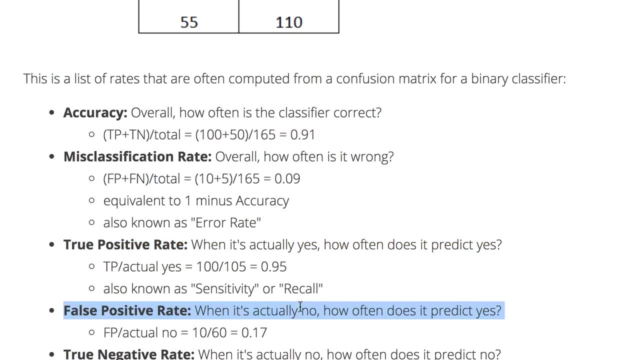 and that's a term that's often used in the machine learning field. So, true, positive rate, sensitivity, recall, all of those are equivalent. Okay, The next term to talk about is called false positive rate, and it answers the question when it's actually no. 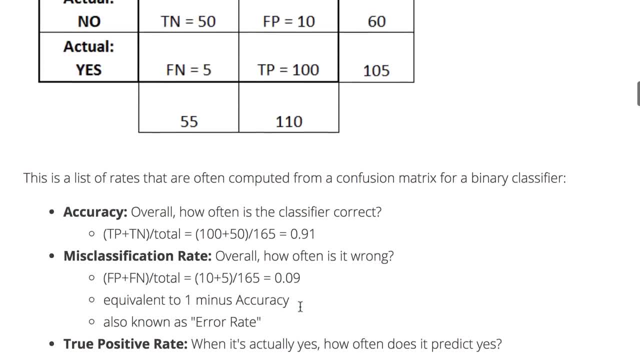 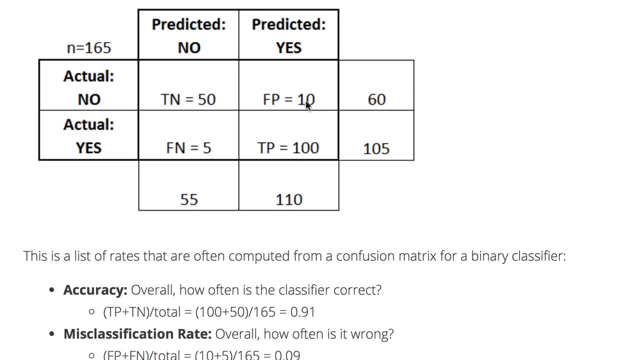 how often does it predict yes So, when it's actually no, 60 cases. how often does it predict yes: 10 cases. So the false positive rate is 10 divided by 60, which is about 0.17.. Okay, 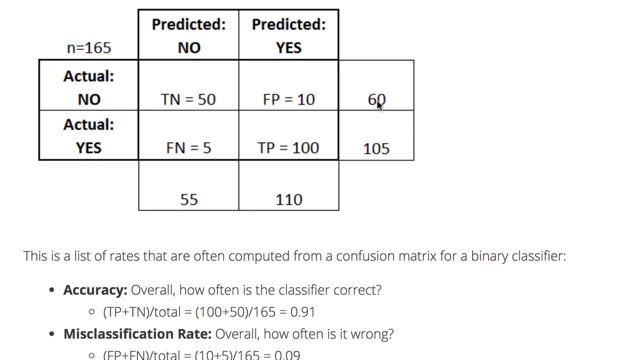 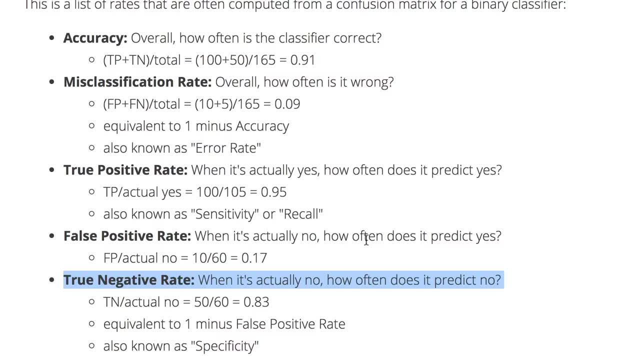 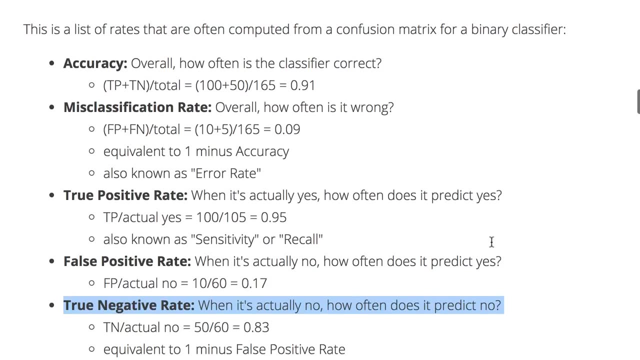 So that is false positive rate. The next term to talk about is called true negative rate, So it answers the question when it's actually no, how often does it predict no? So if we scroll up here when it's actually no, 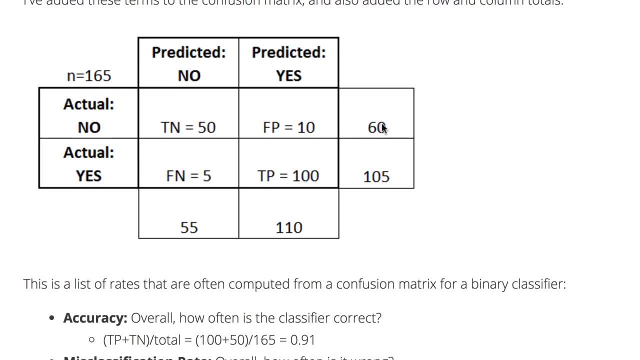 60 cases. how often does it predict no 50 cases? So 50 over 60 is about 0.83.. You may have noticed this is equivalent to one minus the false positive rate, which was 0.17.. And it's often known. 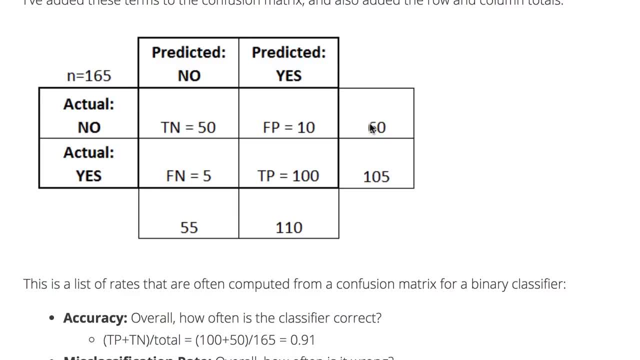 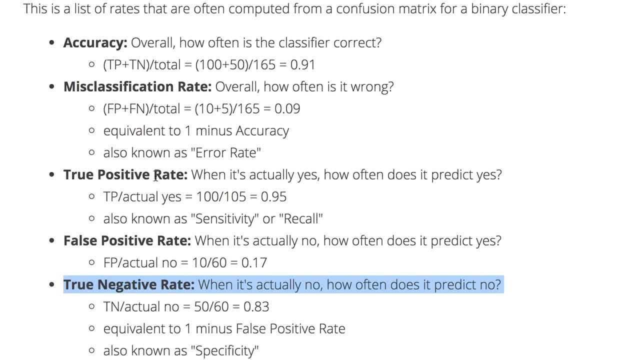 perhaps more commonly known as specificity. Okay, So just to recap here: your true positive rate is also known as sensitivity or recall, And your true negative rate is also known as specificity, And that's probably a more common term than true negative rate. 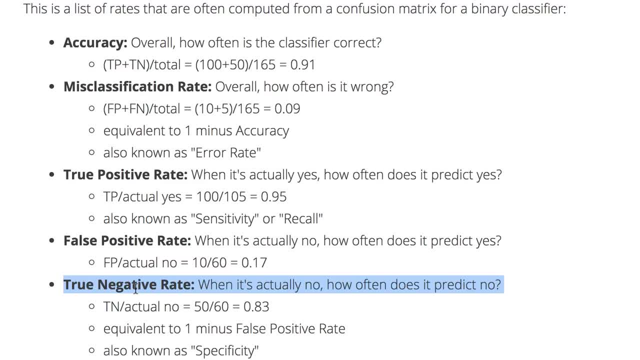 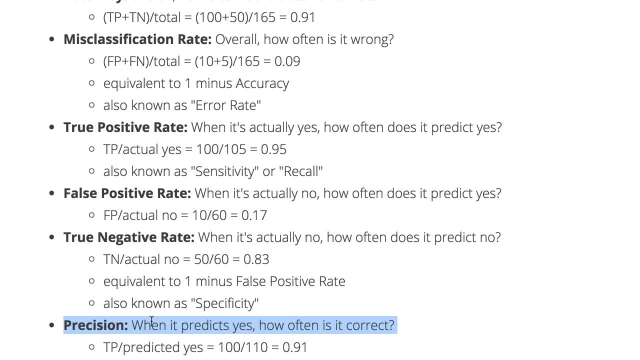 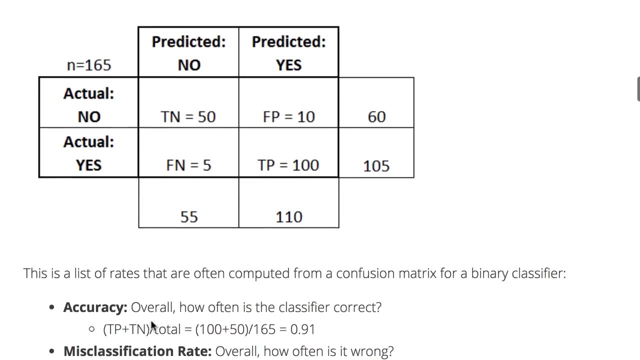 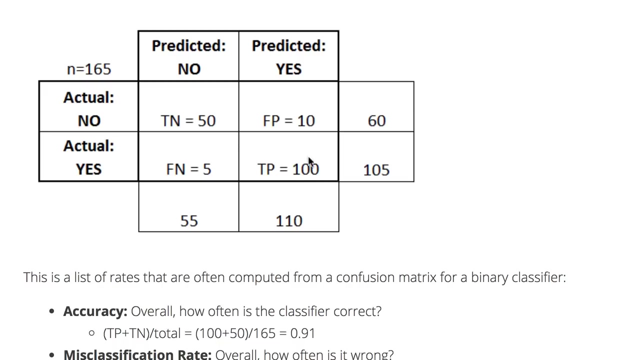 The final term I want to talk about before we get into questions is the term precision, which answers the question. when it predicts yes, how often is it correct? So scroll back up here: When it predicts yes, 110 cases, how often is it correct? 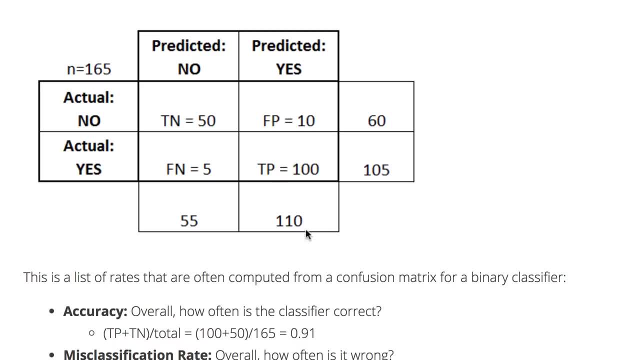 100 of those cases. So it's 100 divided by 110, which is about 0.91.. Now, this is the first rate that we have talked about in which the denominator is one of these numbers instead of these numbers, So it can be a little bit confusing. 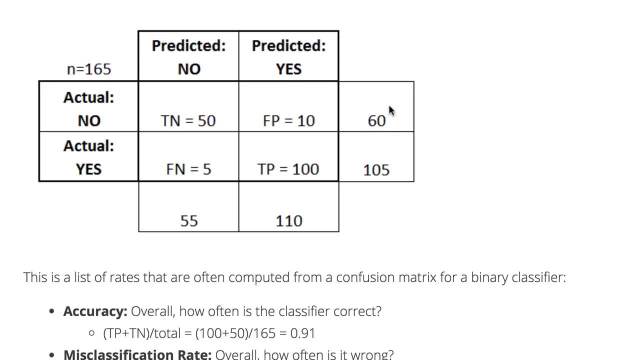 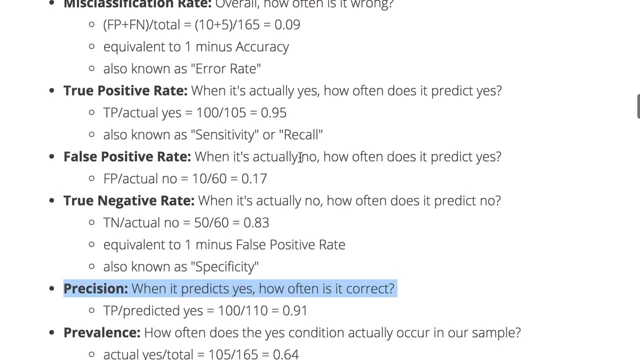 to keep track of, I know, But again, precision answers the question when it predicts yes. how often is it correct? So 100 out of 110.. Now I'm going to go ahead and move down to the questions. I'm going to skip prevalence. 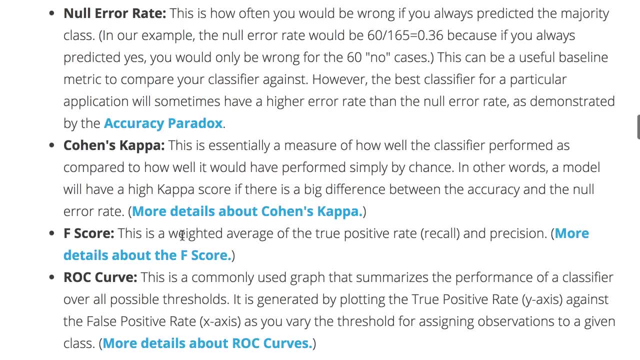 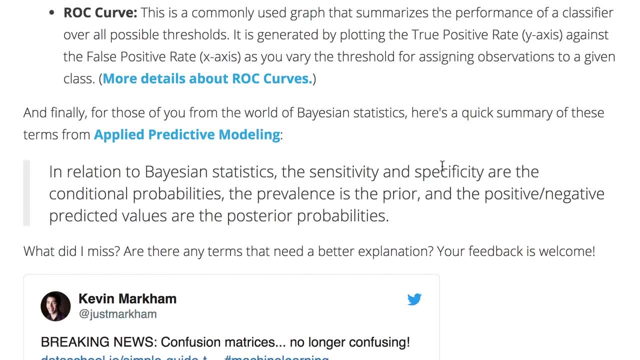 and then some other terms that I've listed down here. You can read about those if you're interested. They're not quite as common. I do want to say one quick thing about the ROC curve. So the ROC curve is generated by plotting the true positive rate. 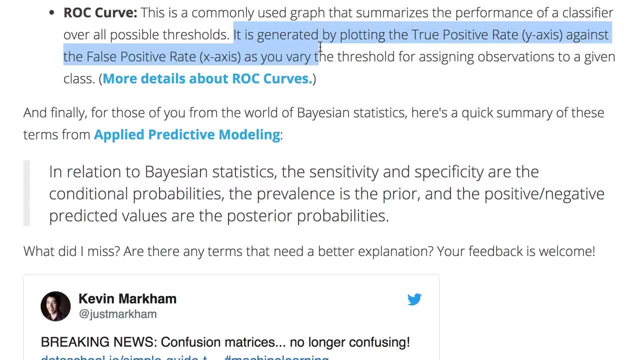 against the false positive rate, as you vary the threshold for assigning observations to a given class. So I mentioned the ROC curve, number one because it's a concept I really enjoy and number two because it's so common. But I do want to say 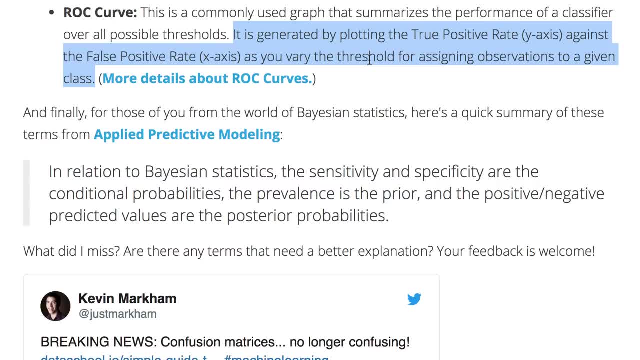 that the ROC curve and the area under the curve cannot be computed from the confusion matrix. You compute that in a totally different process. If you're interested in the ROC curve, I have a link here to a video I made about that. Here's a quick example. 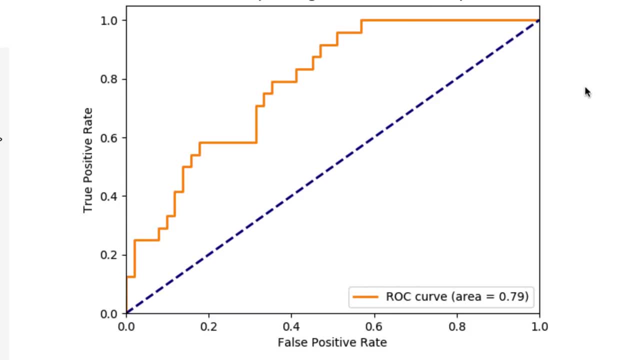 of what an ROC curve looks like. This is from the scikit-learn documentation. There is another similar curve called the precision recall curve, which is, as you might guess, a plot of precision versus recall. And again, that cannot be computed. 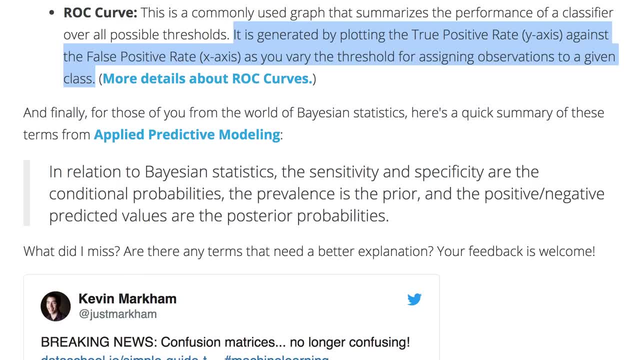 from the confusion matrix. So the ROC curve and the precision recall curve, those are not model evaluation metrics. they are more like tools for model evaluation, in a way similar to how the confusion matrix is a tool for a model evaluation, not a number itself. 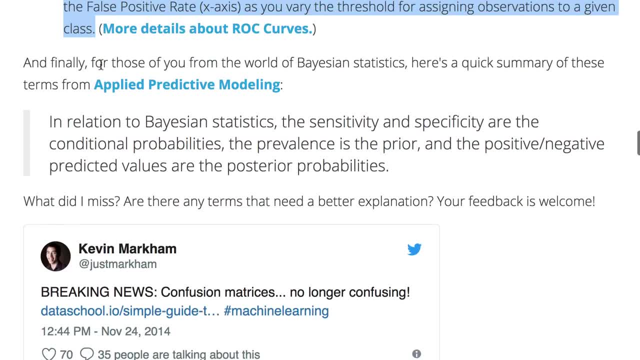 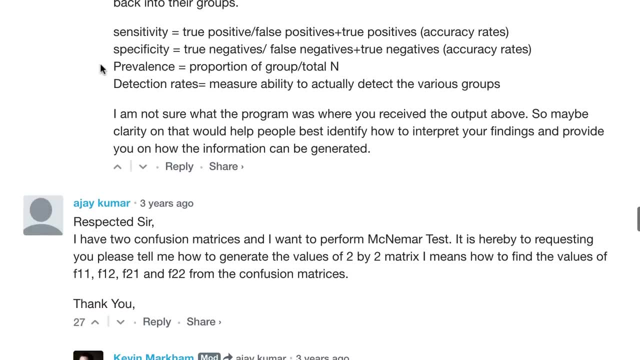 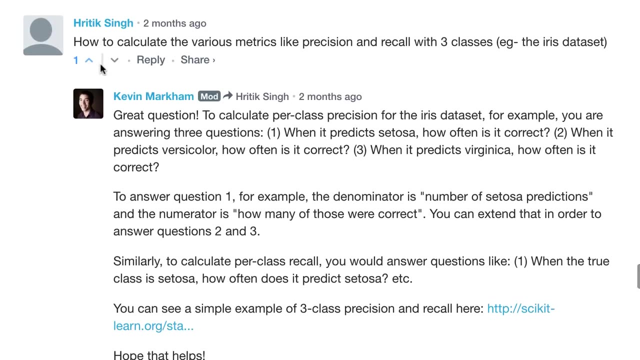 Okay, All right, let's move down to the four excellent questions I've picked out from the comments section that I've received over the years. And here is the first one I want to talk about, And the question is how to calculate various metrics. 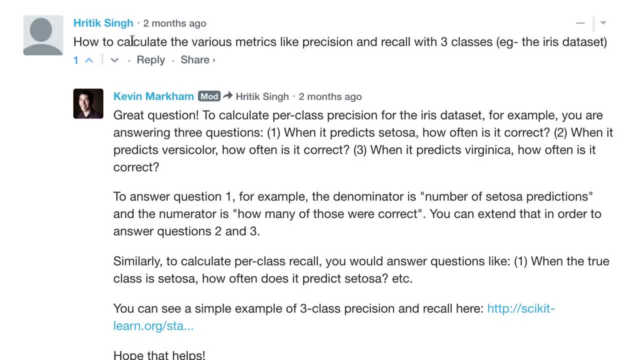 like precision and recall with three classes. It's a great question because the definitions I presented for precision and recall give a single precision and recall for a confusion for any given confusion matrix. So let's scroll up back and take a quick look. 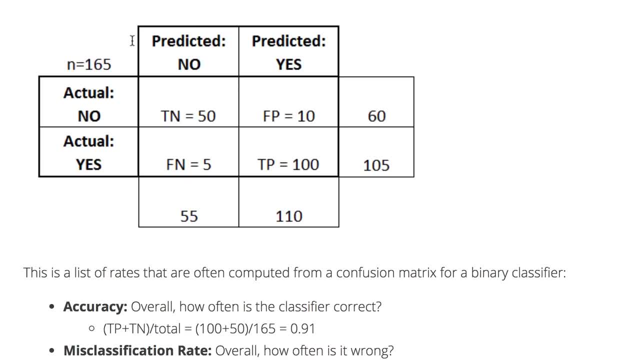 and I can explain how this would work. So recall, as you might recall, recall is when the true value is yes, how often does it predict yes? So 100 over 105.. And precision is when it predicts yes, how often is it correct. 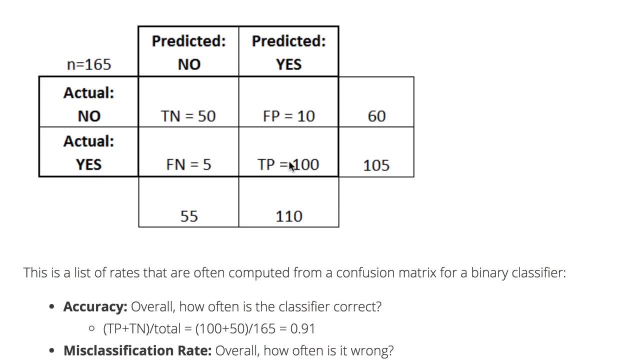 So 100 over 105.. So 100 over 110.. For this confusion matrix, those are the numbers you would call the recall and the precision. Okay, However, you might think to yourself that you could calculate these for the other class. 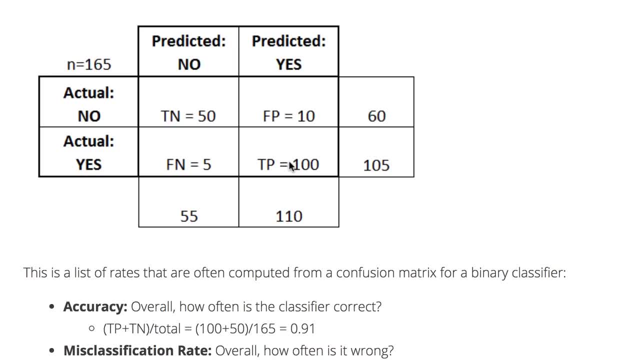 In other words, what's the recall and the precision for the no class? Okay, So the recall would say: when the actual value is no, how often does it predict no? That's the recall for the no class And the precision for the no class is. 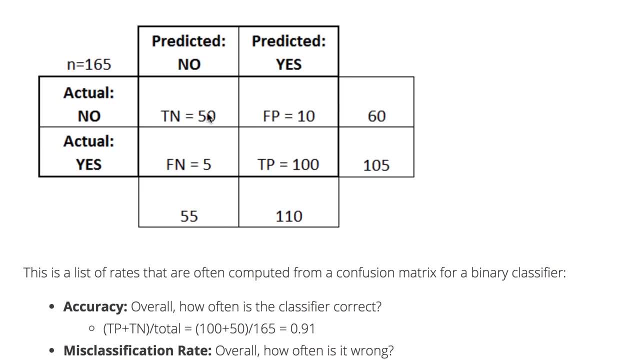 when you predict no, how often is it correct? So, 50 out of 55 for the no class precision and 50 out of 60 for the no class precision. Okay, So I'm gonna show you in a second how to do this for three classes. 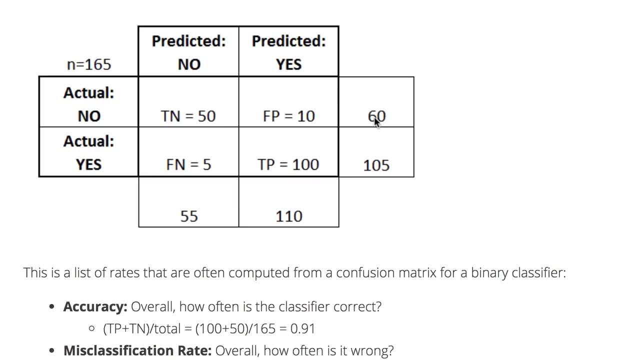 But just to be clear, if you have a binary problem, meaning one with two classes, and someone asks you for the recall or the precision, they are asking you about the recall and the precision for the positive class, and that's the convention. 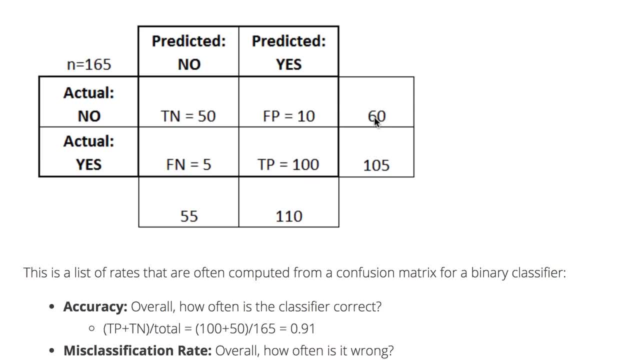 But you can compute the recall and precision for any class. Okay, So, as I just showed you, you can compute the recall and the precision for the no class, for the negative class. Okay, so let me show you this example of three classes. 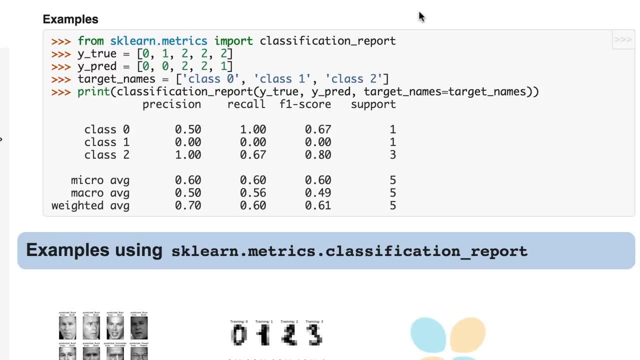 And this is from the scikit-learn documentation for a function called classification report And in this three class example, scikit-learn calculates the precision and the recall for each of three classes. So let's do a quick example And the thing you have to understand: 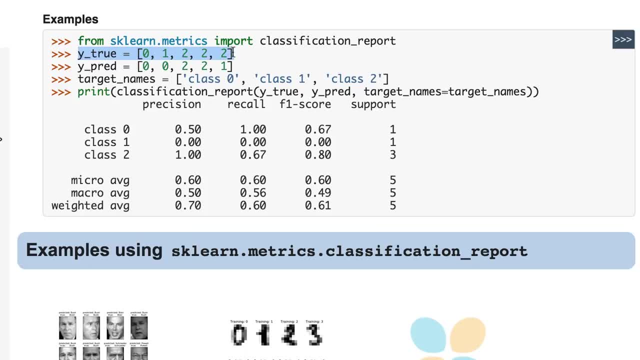 is that, in this case, here are five true values and then here are the five values predicted by a classifier. Okay, So you see that it was right: one, two, three out of the five times, Thus you would say, the accuracy. 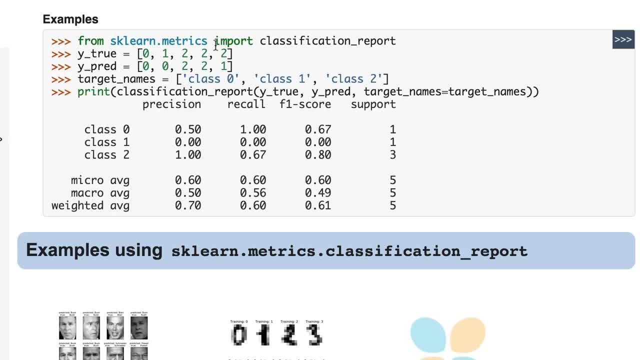 was three out of five or sixty percent. Anyway, let's talk about computing the recall and precision for one of these classes. Alright, So we'll take class zero. Well, what's the recall for class zero? So recall means when the true value is zero. 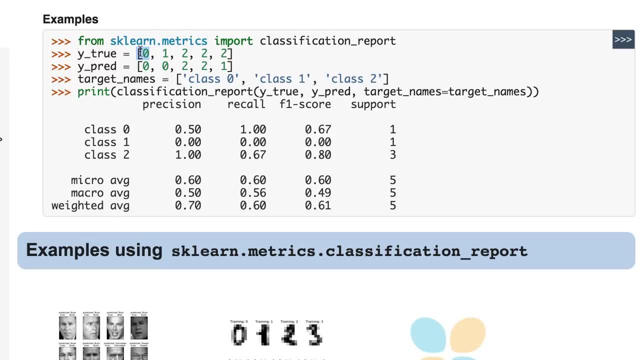 so this is the recall for class zero, when the true value is zero. how often did it predict zero? One hundred percent of the time, Which is why the class zero recall is one or one hundred percent. The precision is when it predicted zero. 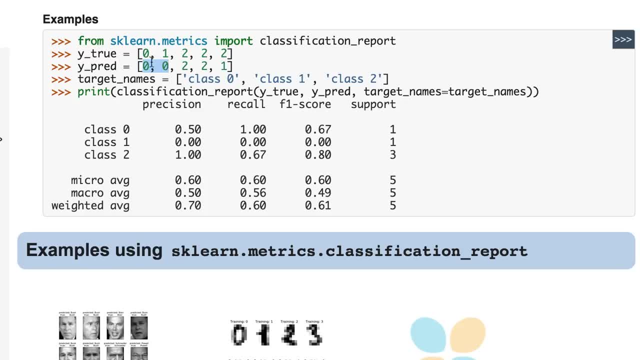 how often was it correct? And the answer is fifty percent of the time, Which is why the precision for class zero is fifty percent, And you can see that you can use that same exact process to compute the precision and recall for each of the three classes. 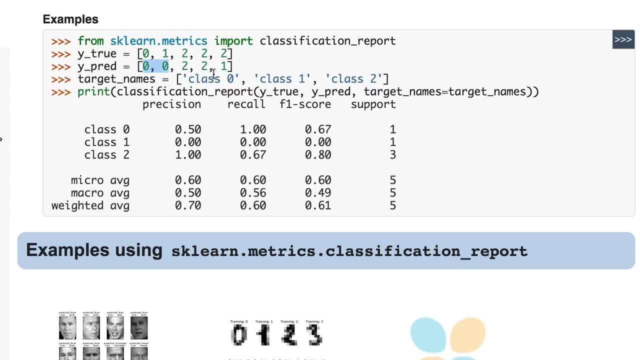 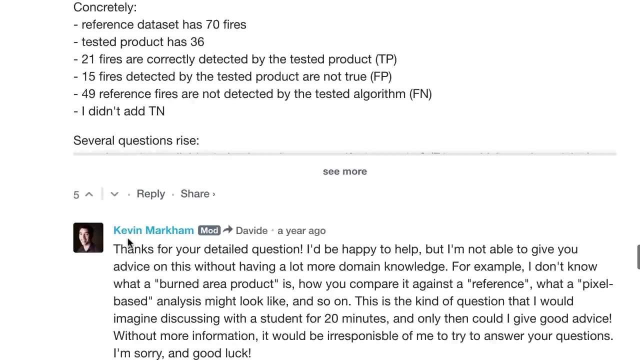 This is one reason that precision and recall are really popular for multi-class problems in machine learning, because you can compute recall and precision for every single class. Alright, let's move back to the questions, and I will take another question out of here and answer it. 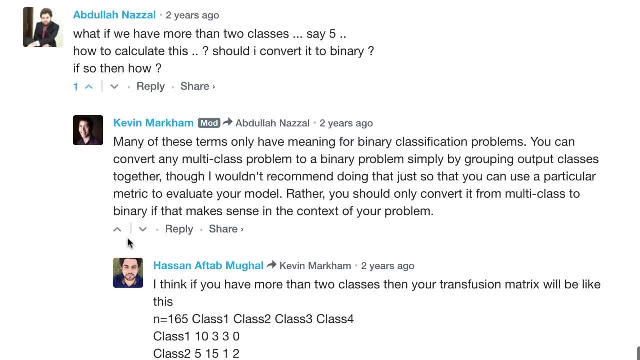 Sorry for all the scrolling. Alright, here's the next question. What if we have more than two classes, say five classes? how do we calculate this? Okay, so what does it look like to have a confusion matrix with more than two classes? 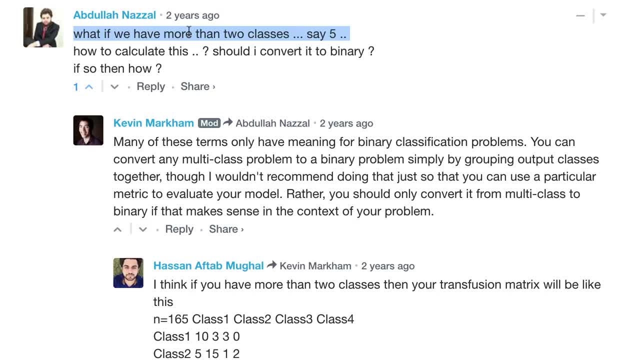 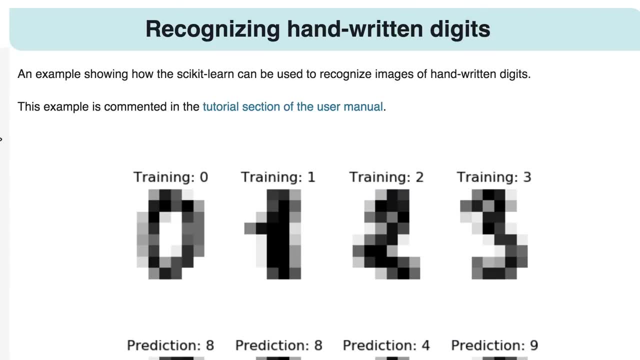 So I'm going to pull up a ten class confusion matrix from the scikit-learn documentation. This is an example of recognizing handwritten digits. In other words, the data is handwritten digits that have been digitized and then some sort of machine learning model. 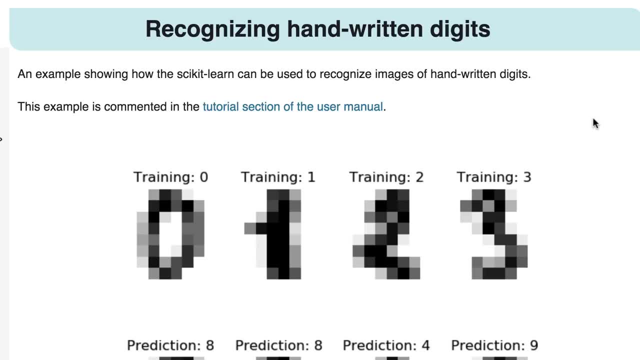 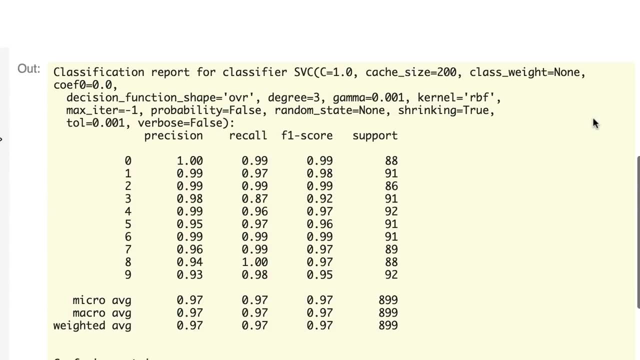 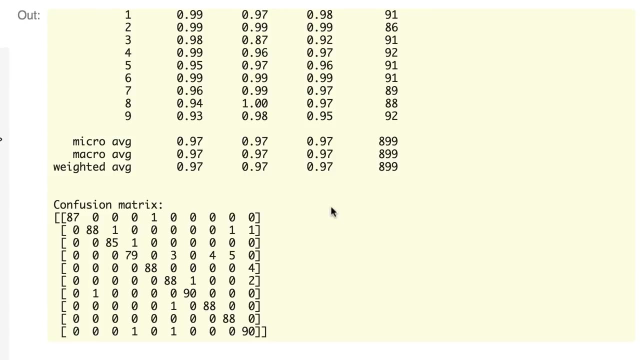 is trying to decide which of the ten digits each drawing represents. So I'll scroll down and this is the confusion matrix for this ten by ten problem, for this ten class problem. As you can see, it's not labeled, but the true values. 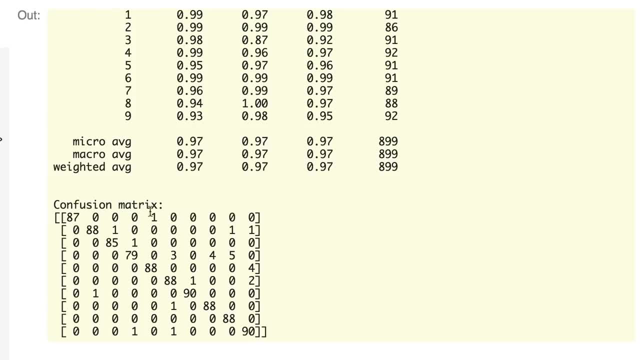 are on the left and the predicted values are on the top. So, in other words, this row is true values zero, and I'll just say: true values zero one, two, three, four, five, six, seven, eight, nine. 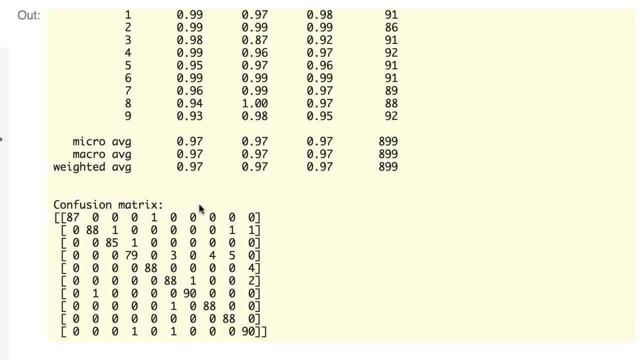 And then the predicted values zero, one, two, three, four, five, six, seven, eight, nine, And with scikit-learn they always just put those in alphabetical order or numerical order, starting in the top left. So you can see that the diagonals. 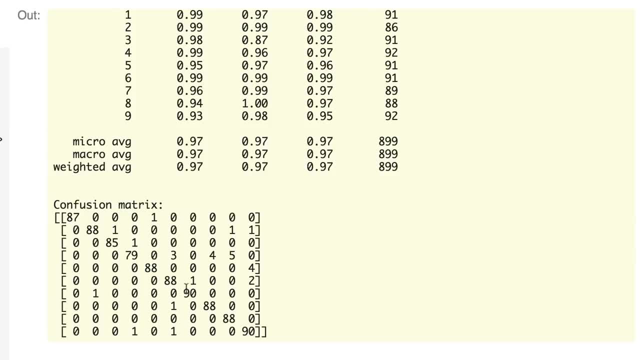 are all the correct predictions, all right. So obviously this model is doing pretty well because all of the big numbers are on that diagonal. And just to take an example, let's pick out this number, this five, which is the largest number. 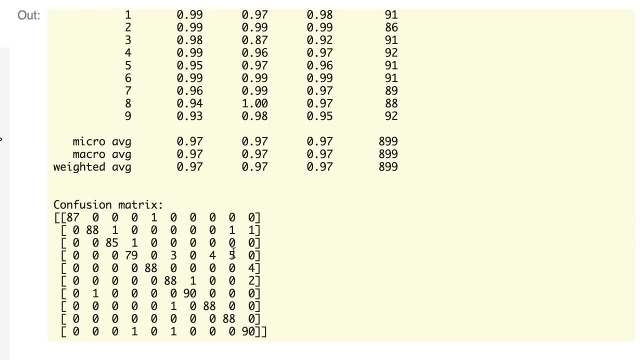 not on the diagonal and talk about what that means. So that means the actual value of zero one, two, three and a predicted value, one. sorry zero one, two, three, four, five, six, seven, eight. 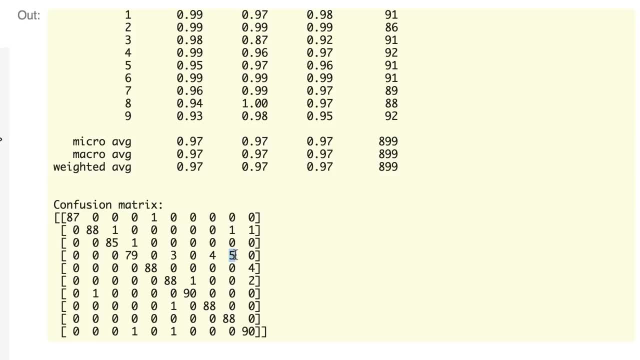 So this five represents five cases in which the actual, the true value was three and the predicted value was eight. Now, that was the most common error and it makes intuitive sense, because a three looks a lot like an eight. okay Now, conversely, 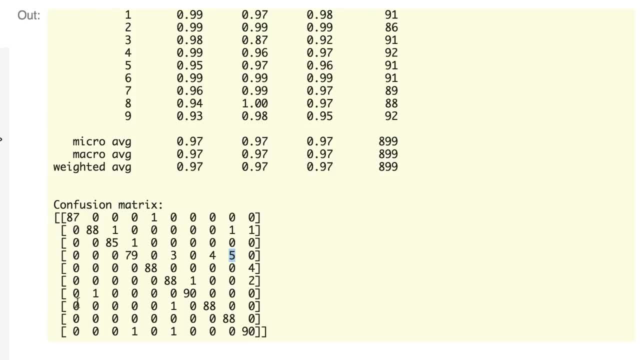 let's look at the case of eights, which is this row being predicted as threes, And it turns out that, with this particular model and this particular data set, eights never got predicted as threes, Maybe because when you've got 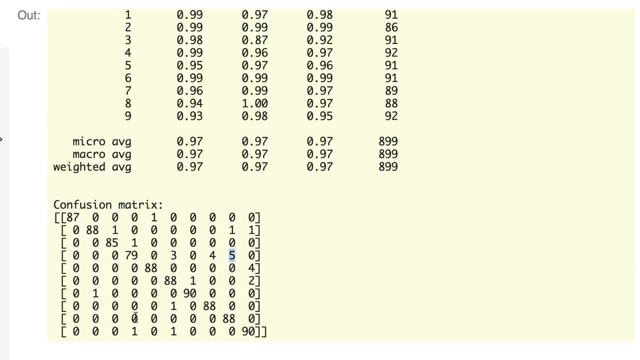 that shape of the eight, it's really obvious to the model that it's an eight, whereas when it's a three, which obviously that's not handwritten but as a three, it's not as clear. like: oh, is that circle kind of filled up? 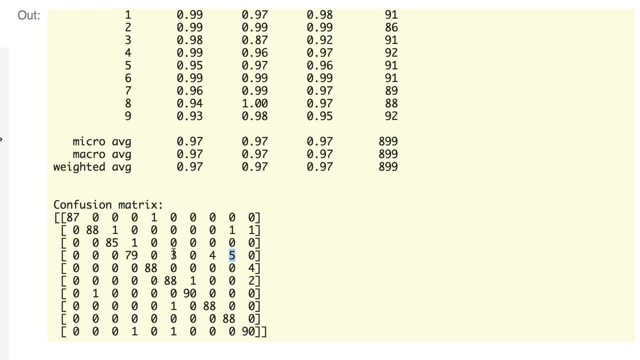 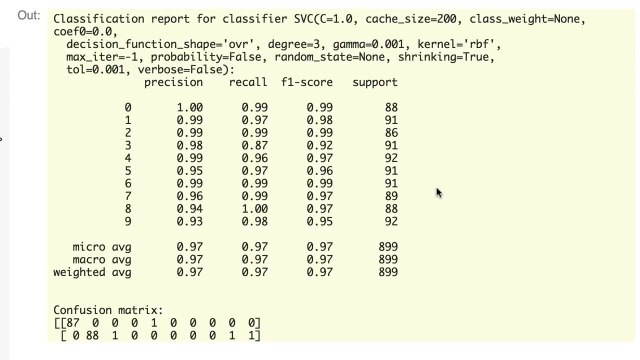 such that it should be counted as an eight. So if you look at the classification report for this particular model, you'll see that threes have the worst recall- okay, which makes sense- whereas eights have perfect recall, And we knew that without even. 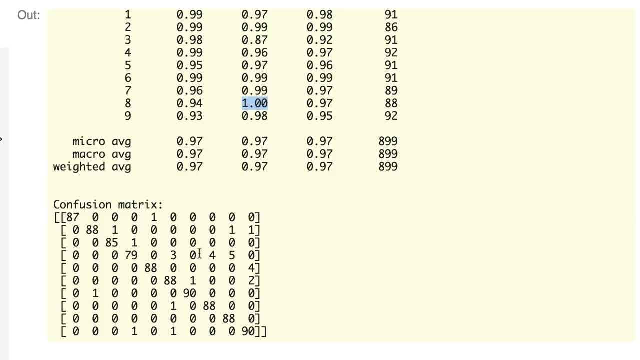 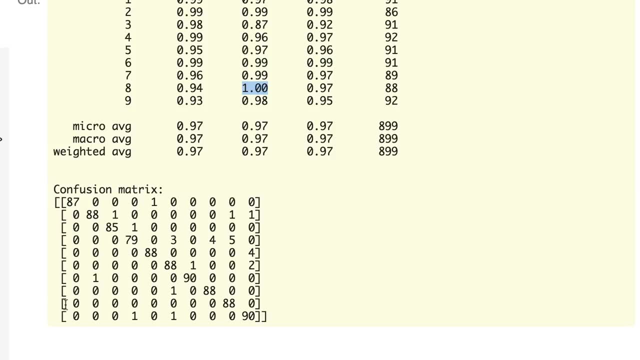 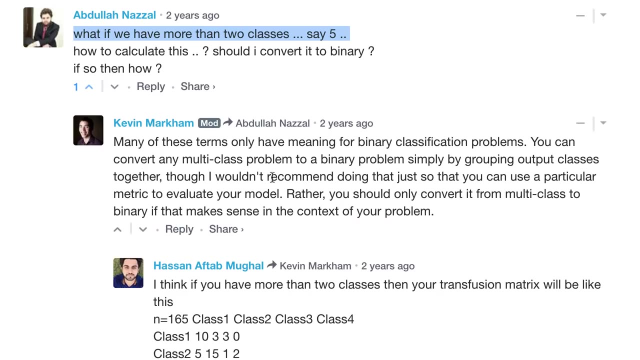 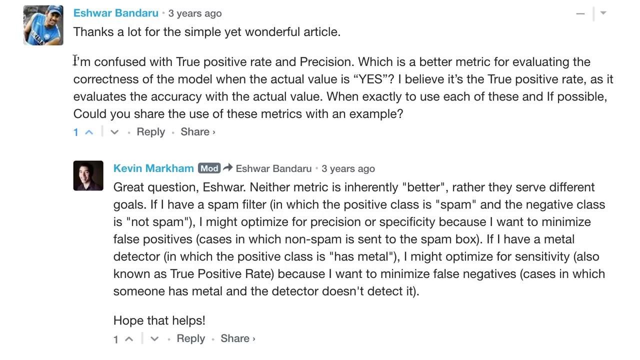 looking at the classification report, because threes have all these errors, whereas eights have no errors. okay, All right, hope that was helpful. Let's move back to the third question I chose, which is right here, And he says: I'm confused with true positive rate. 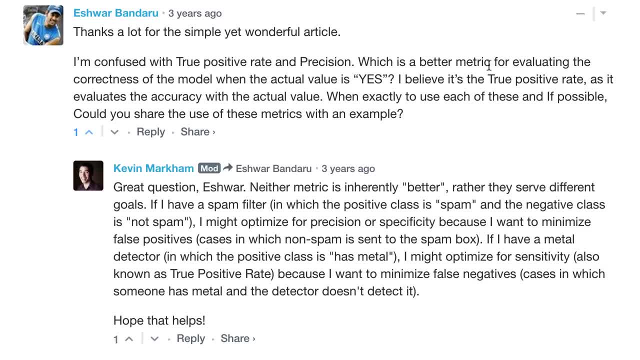 and precision. which is a better metric for evaluating the correctness of the model? Okay, great question. So he's correct. He's correct that to choose between models, you do have to focus on an evaluation metric, But the question is, what metric should you focus on? 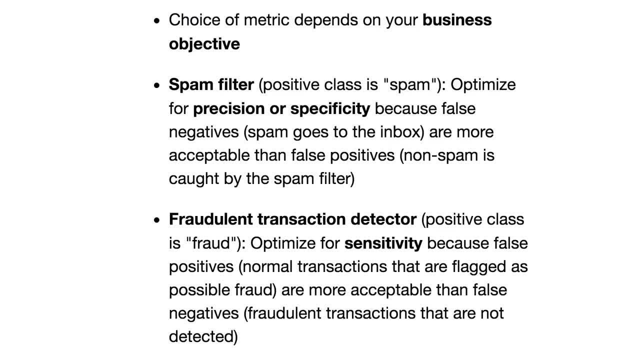 So to answer that, I'm going to pull up the Jupyter Notebook from a video I made about classification classifier evaluation using scikit-learn in Python, And I just want to talk about this for a minute. So your choice of which metric to focus on. 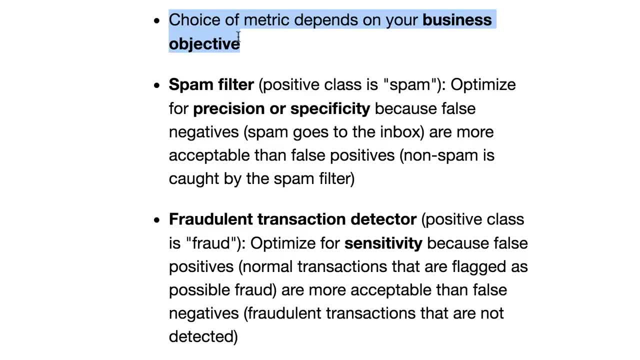 depends on your business objective. So, for example, if you are building a spam filter in which the positive class is spam, you might choose to optimize for precision or specificity. Now, why would you do that? Well, you would do that because false negatives. 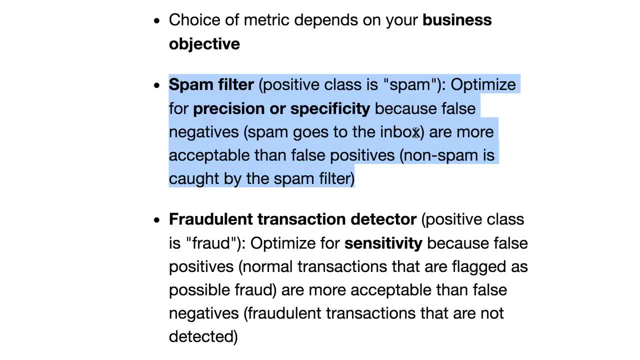 meaning spam goes to the inbox again. the positive class is spam, so a false negative is when spam does not get flagged as spam. False negatives are more acceptable than false positives, which is when non-spam is caught by the spam filter. 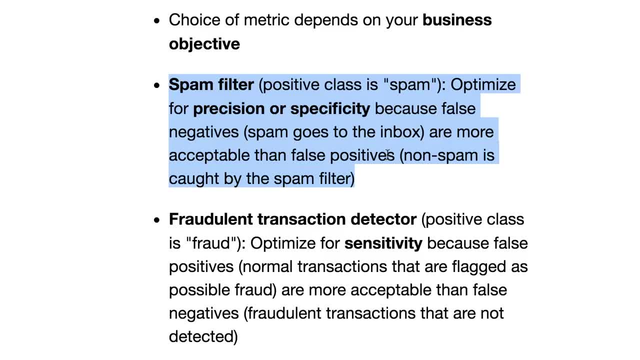 And you would agree. it's not that annoying to occasionally get some spam in your inbox, but it's super annoying when a piece of real email that you need to receive is in your spam filter and you never notice for a month, because that's when you check your spam filter. 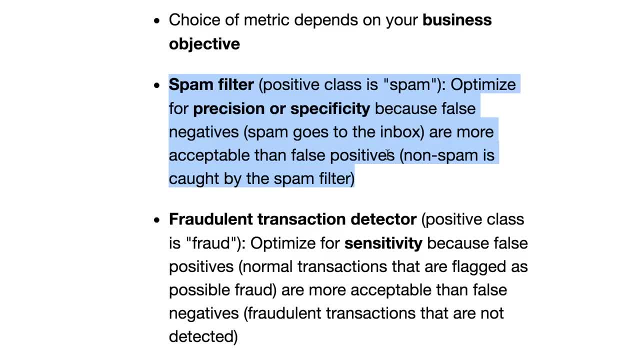 So ultimately, we're making a value judgment about which errors to minimize and choosing an appropriate metric to match that judgment. Now, just to give you a different example: if you were building a fraudulent transaction detector in which the positive class is fraud, you might optimize instead. 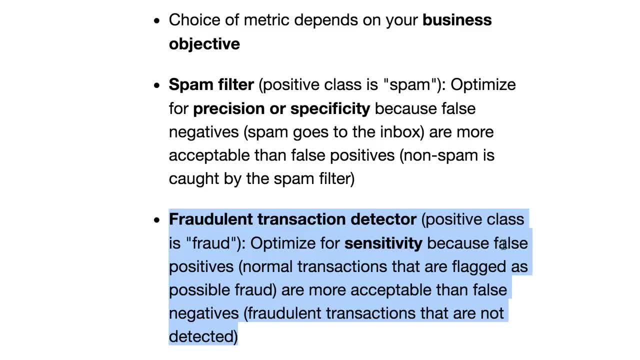 for sensitivity, because false positives, meaning normal transactions flagged as possible fraud, are more acceptable- well, at least depending on your viewpoint- than false negatives, fraudulent transactions that are not detected. So again, you're looking at your business objective and you're choosing. 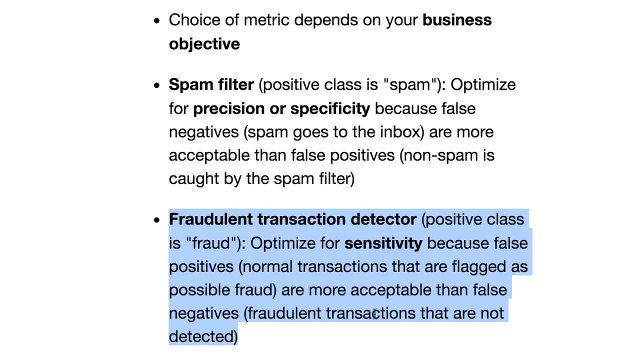 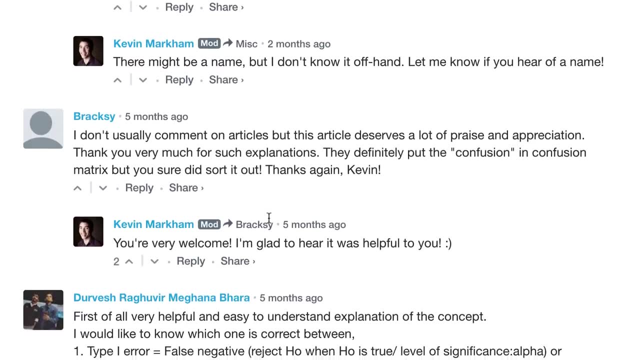 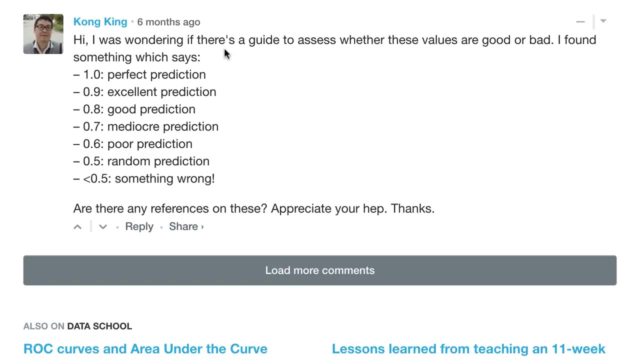 the appropriate evaluation metric based upon what type of errors you are trying to minimize. okay, All right, let's move back to the final question that I will go through. All right. So the question here is: I was wondering if there's a guide. 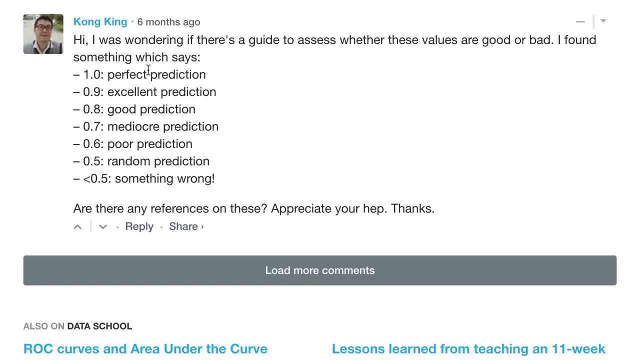 to assess whether these values are good or bad, I found something which says 1.0, perfect prediction, 0.9, excellent, 0.8, good, 0.7, mediocre, etc. etc. Now I assume that these numbers 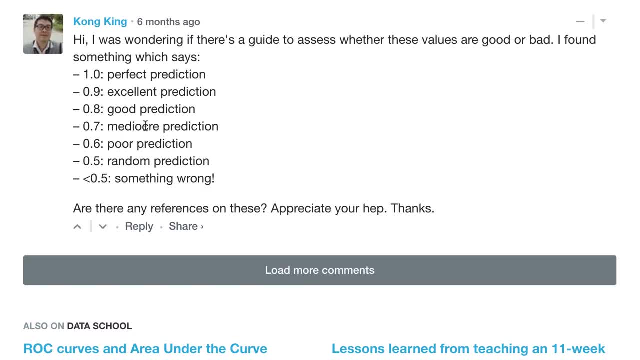 are the accuracy scores for a binary classification problem. I assume that's what these are supposed to represent. If I'm correct about that, I would say that these descriptions- perfect, excellent, good, based upon the number- are useless. They are completely useless. 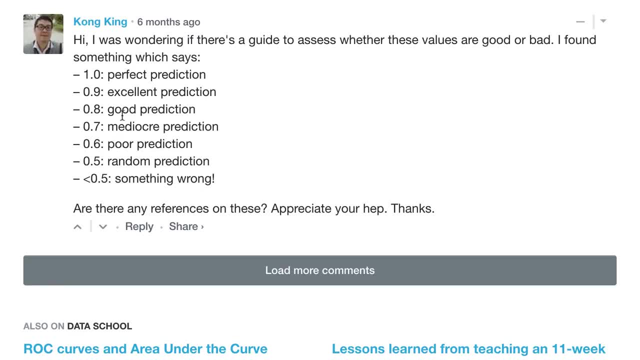 And here's why. okay, Let's pretend that a credit card company hired you to build a detector of credit card transactions that are fraudulent. If you built something for them and it had 90% accuracy, they would probably fire you because 90% accuracy. 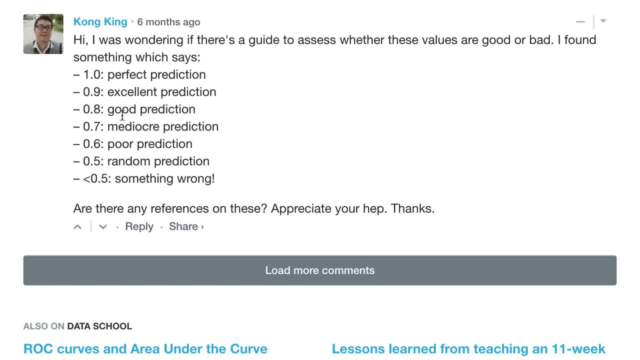 is not good. Why is it not good? Because let's say that 1% of transactions are fraudulent, You can get a 99% accuracy without any work at all by always predicting that it's not fraud. So again, this is known. 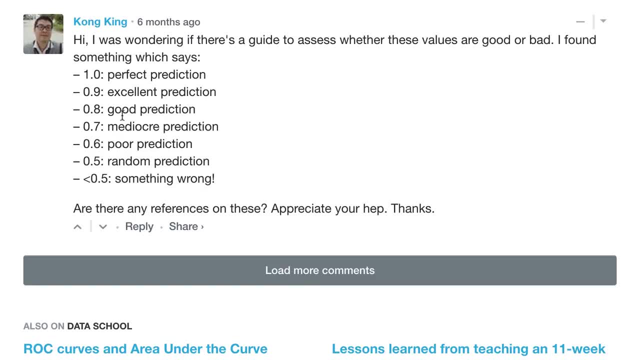 as class imbalance. okay, When you have a significant imbalance in your classes, in your class labels, and one would expect that most transactions are not fraudulent. So you know what accuracy would be good for a fraudulent transaction detector if only 1% of transactions. 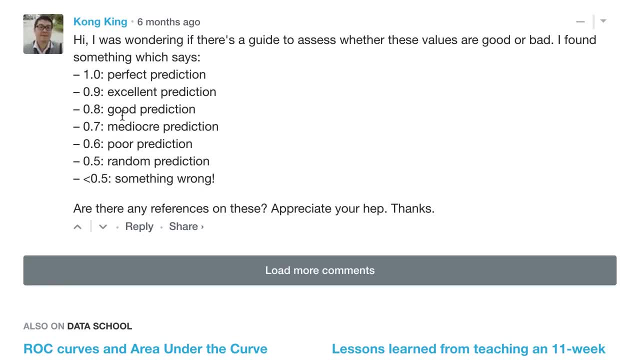 are fraudulent, Maybe 99.9.. I don't know. You'd have to ask the company what they consider good, But it's certainly not that 90% is excellent. okay, Now let me give you a different example. Let's say you're in.